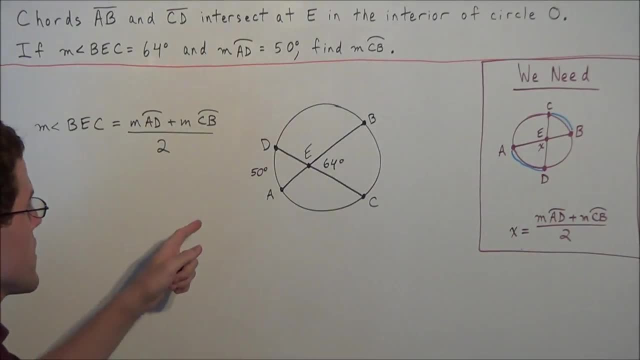 for the two pieces of information that was given to us. That is, we know that the measure of angle BEC is equal to 64 degrees, So we can replace this piece here with 64 degrees, And now we can set this equal to. the measure of arc. AD is equal to 50 degrees, So now we 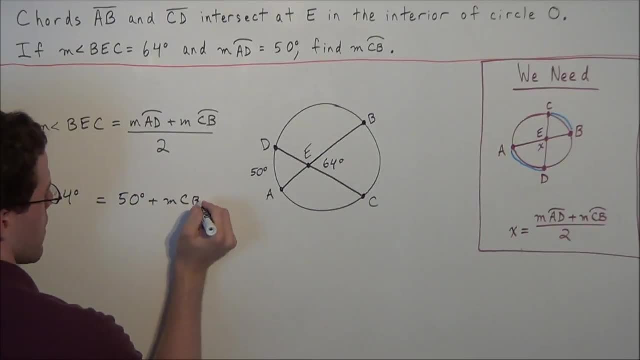 have plus the measure of arc CB divided by 2.. So now to solve for the measure of arc CB, all we need to do now is cross multiply, So we could call this 64 degrees divided by 1.. And now we have 2 times 64 degrees, That's 128 degrees equals. And now we have 1 times. 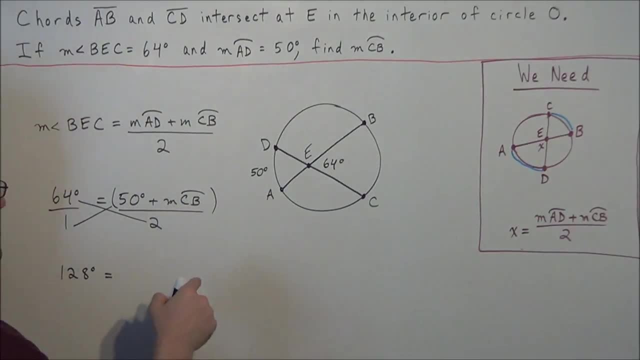 50 plus the measure of arc CB. But 1 is the identity element of multiplication. So we could just rewrite this expression here And we have 50 degrees plus the measure of arc CB. So now to solve for the measure of arc CB, we'll just rewrite this equation over. 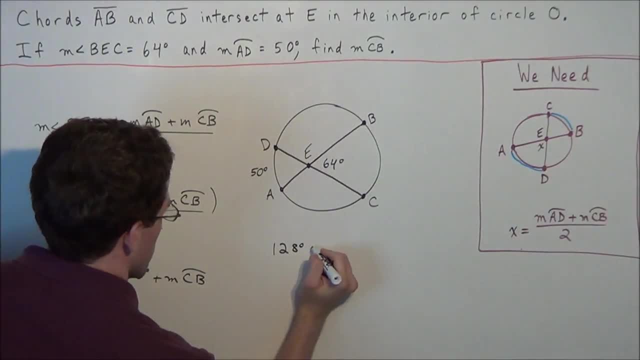 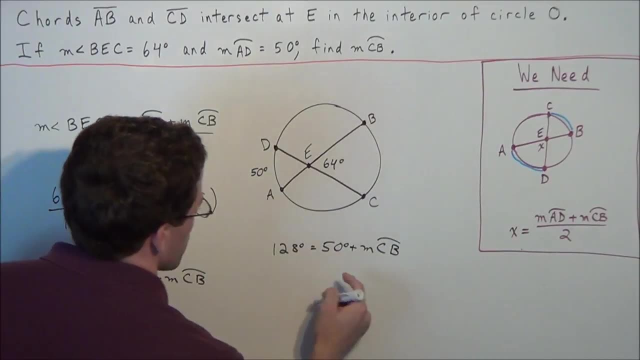 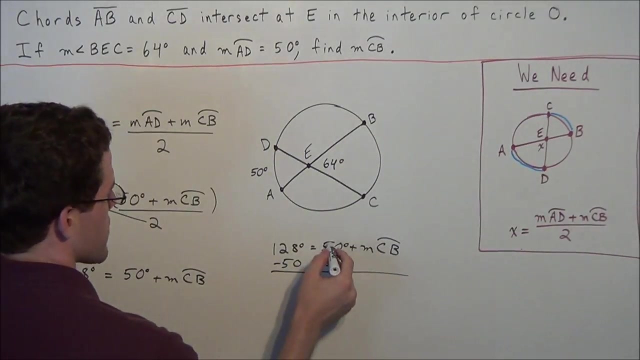 here. So we have: 128 degrees equals 50 degrees plus the measure of arc CB. We just need to subtract 50 from both sides of this equation. So then now we have our answer: 50 degrees minus 50 degrees will cancel. We just got to put these units of measurement. They are: 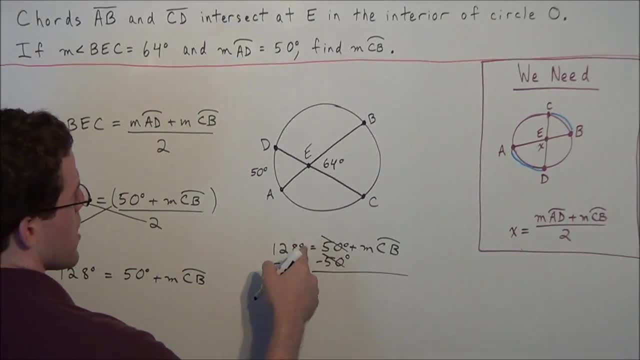 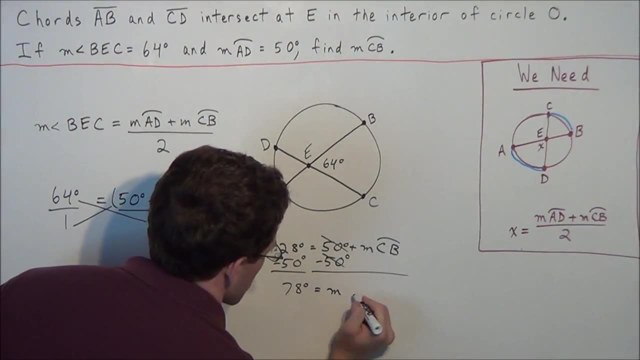 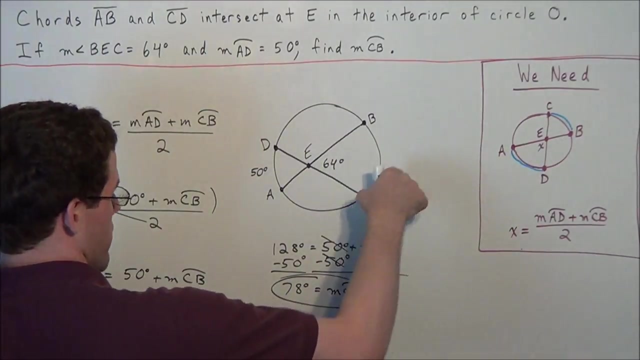 important. So this gives us 128 degrees minus 50 degrees, gives us 78 degrees plus the measure of arc CB. So 78 degrees is equal to the measure of arc CB. So now we could just label this on the circle diagram that we have here. The measure of arc CB is equal to 78 degrees. So just 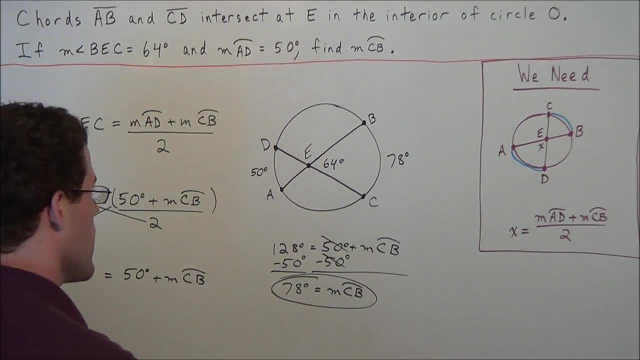 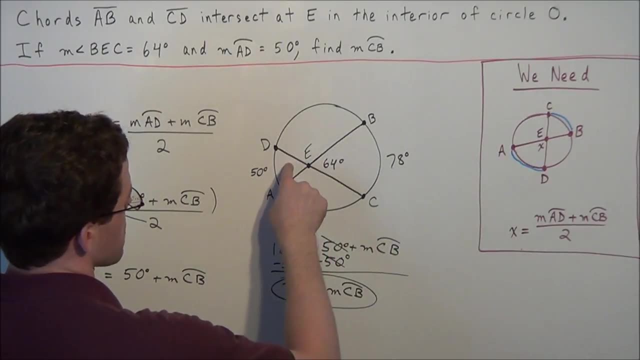 remember, just to recap the way we want to make use of this theorem, we were given the measure of angle BEC. In some sense we do know that the measure of angle AED is also 64 degrees, because these two are vertical angles, So the two arcs that are sectioned, 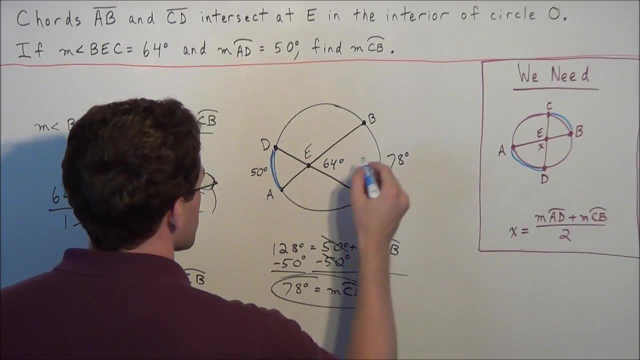 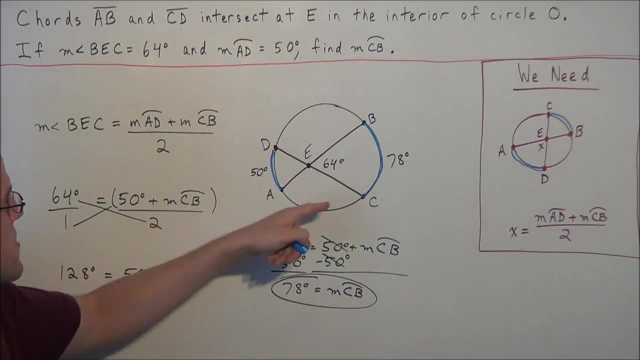 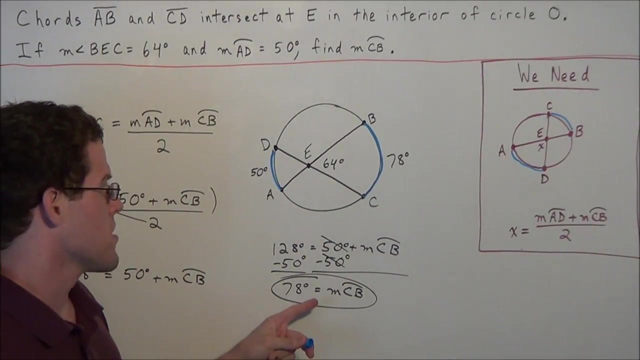 off were arc AD and arc BC. That's why, when we set up this equation, we said the measure of angle BEC was equal to the sum of these two arcs, AD and CB, divided by 2, and we arrived at our answer: the measure of arc CB.